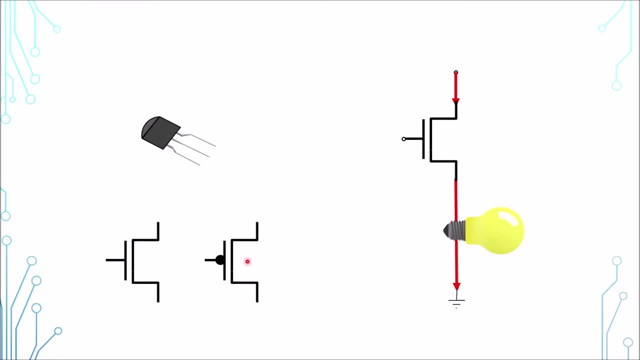 One that is turned on by sending a logical 1 voltage and the other one which is turned on by sending a logical 0 voltage. Now we can arrange several transistors together to perform some basic logical functions. Take a look at the leftmost arrangement. 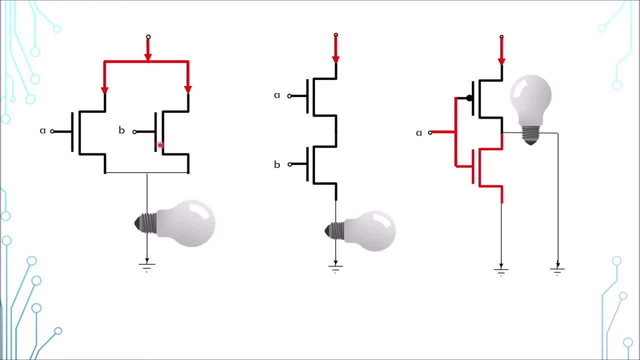 The transistors are arranged in a parallel manner. In order to turn on the load, you can turn on transistor A or transistor B, or both. This forms a logical OR gate At the middle arrangement. the transistors are arranged in a serial manner. 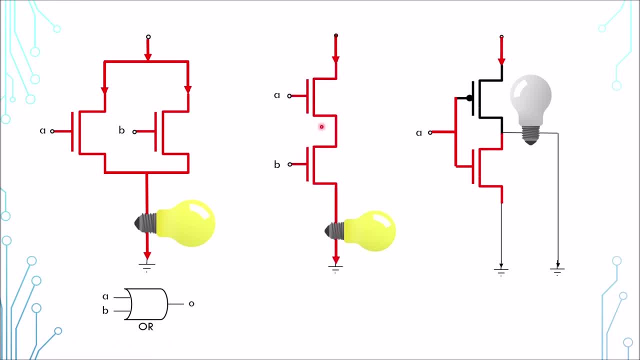 Both transistor A and transistor B need to be turned on for the electric current to pass through. This forms a logical N gate. In this arrangement, two transistors of different polarity are used and they are controlled by the same input of A. 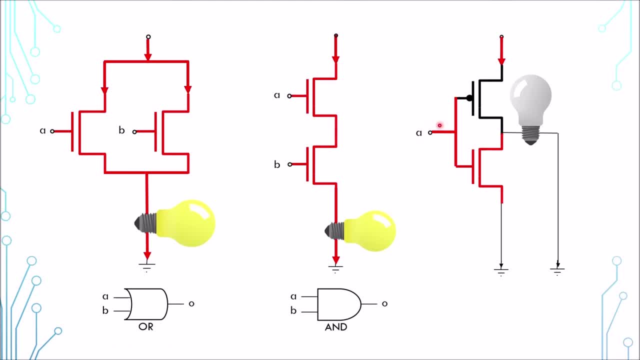 Only one of them can be turned on at one time. The load is turned on if input A is at logical 0 voltage. This forms a logical, NOT gate. Using logic gates, we can combine them to perform even more complex functions. The diagram shows a multiplexer or, in simple English, a selector. 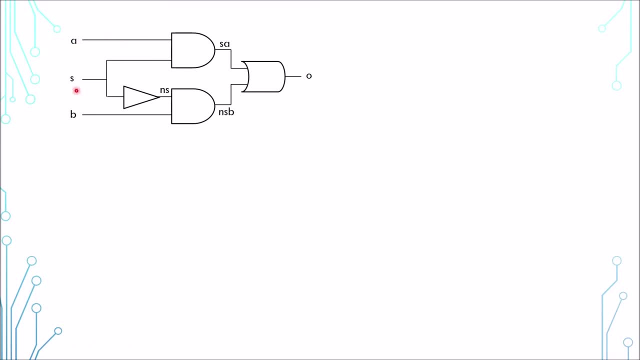 Its output O will follow input A or input B, depending on selector input S. And now, at long last, we've come to system relog. This is to answer the first question. what is system relog? System relog is a hardware description language. 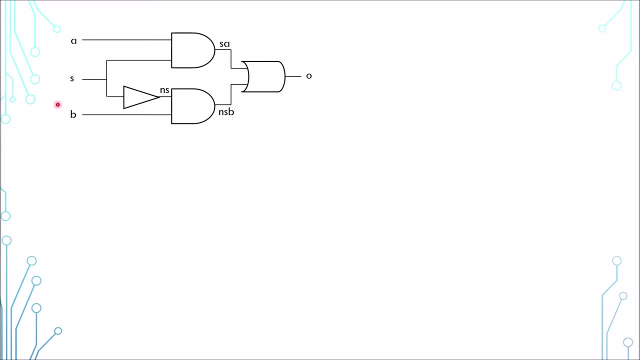 It is capable of describing digital electronic circuit like the one in the diagram. First you use module to represent the design. You provide a name for the design. In this case it is called Mux, which is a shorthand for multiplexer. 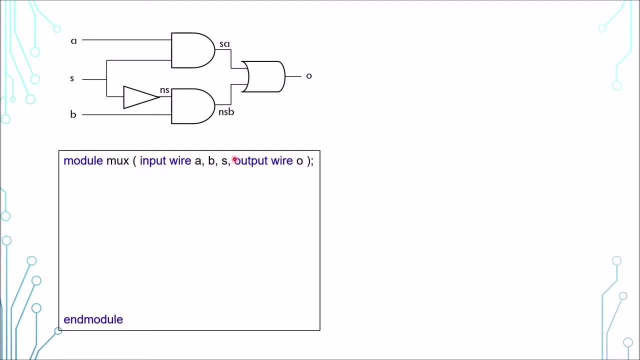 You describe its port in the bracket, which are three input ports A, B and S and one output, port O. There are three internal wires here, here and here. The rest of the code is to connect all the wires together. 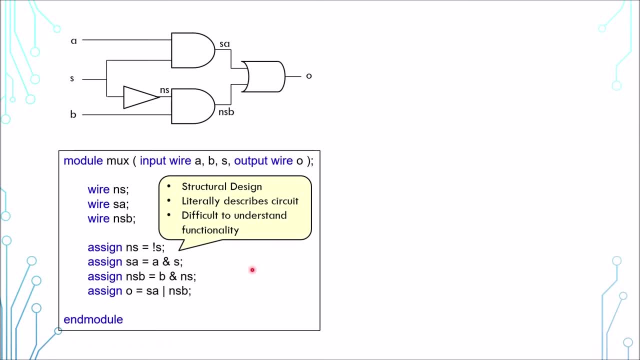 This coding style is called structural design. It is literally describing the circuit gate to gate, connection to connection. The downside of this code is that it is difficult to understand what the design intention is, Which is why there is another way of describing the same circuit.